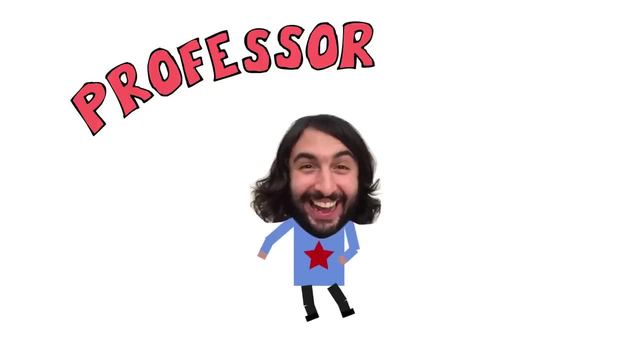 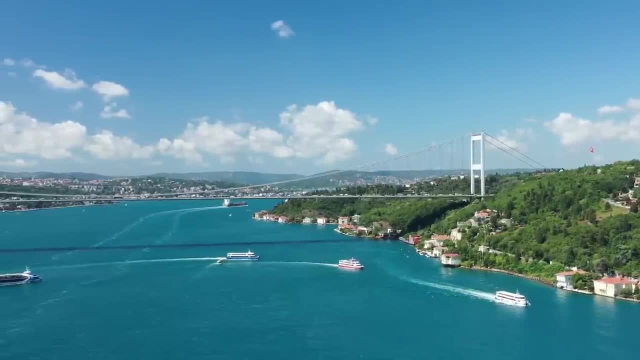 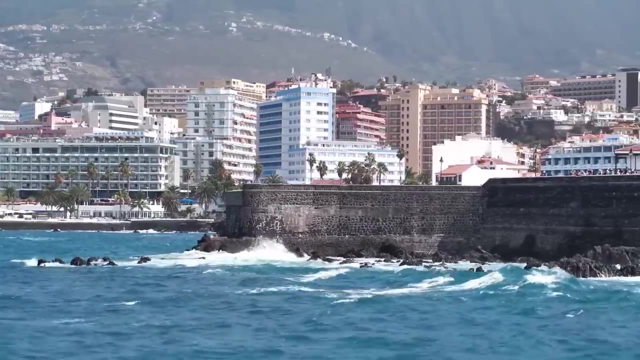 We often think of Earth's surface as a well-explored place that is thoroughly colonized by humans. To some, it may seem as though we know all there is to know about this land we inhabit. However, the truth is that most of the surface of our planet is unexplored due to it being 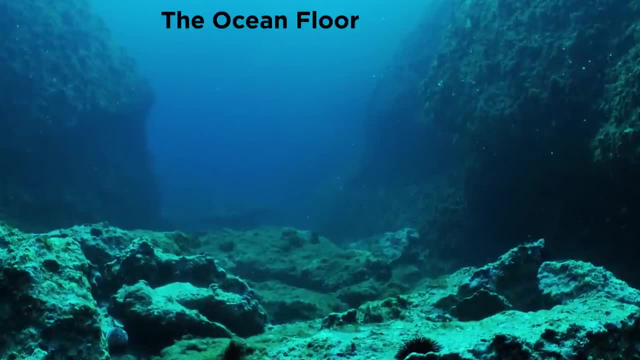 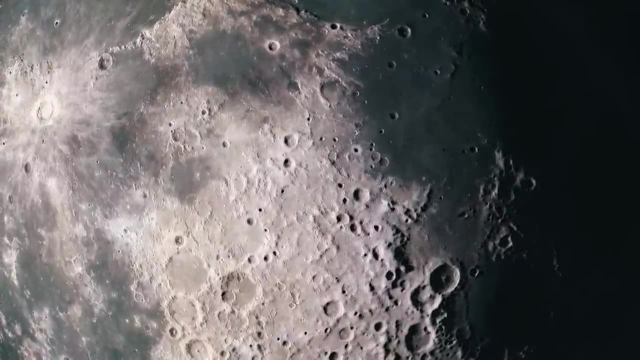 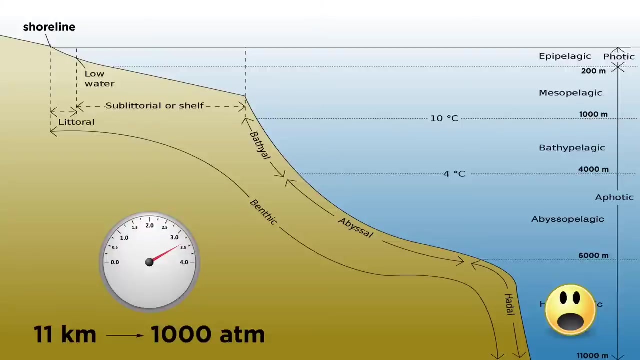 covered with kilometers of water. Of course we are talking about the ocean floor. It sounds crazy, but we know more about the lunar surface than we do about the ocean floor. So why is the ocean floor so difficult to explore? The primary difficulty is withstanding the high pressures that result from the weight. 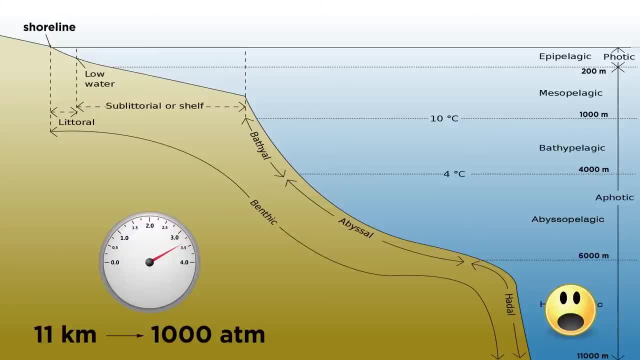 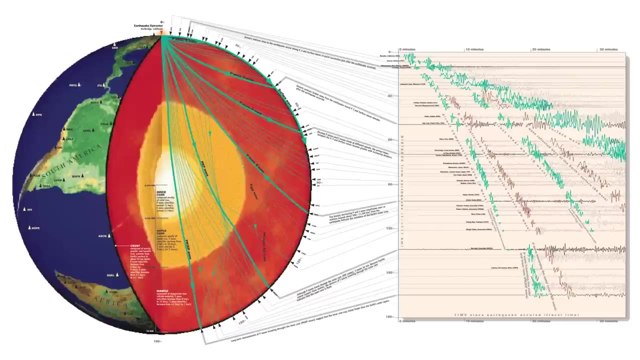 of up to eleven kilometers of water, yielding pressures of more than one thousand atmospheres. Though the deepest areas of the ocean trenches only represent a small area of the ocean, its average depth is still a substantial 3.5 kilometers. But as we know from studying Earth's layers, we do not have to visit an area of the Earth. 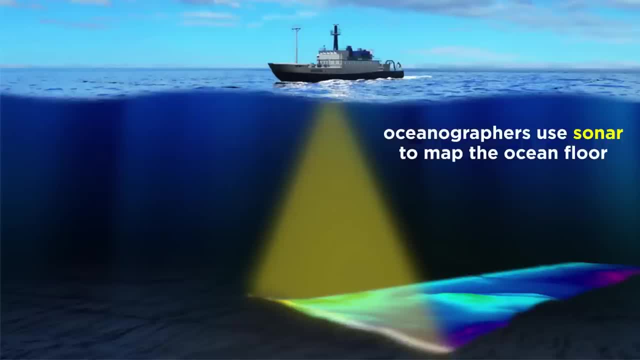 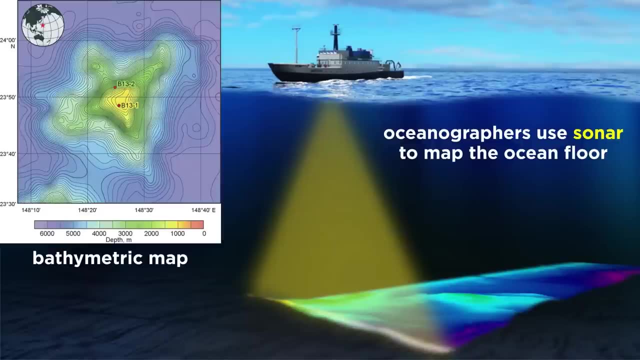 to know something about it. Oceanographers use methods like sonar, which reflects sonic waves off the ocean floor, to determine its topography and create detailed bathymetric maps. Instruments called echo sounders emit a sound pulse and then measure the amount of time. 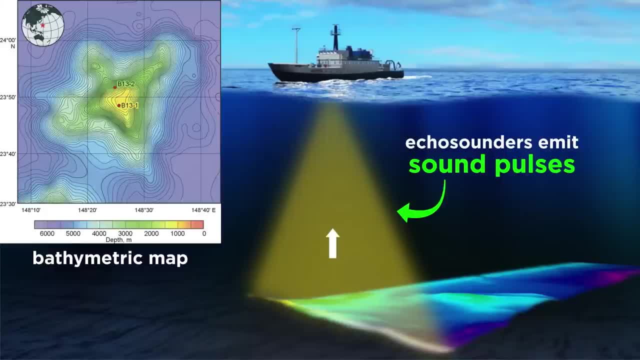 it takes the pulse to reach the ocean floor, bounce off of it and return to the surface. This is a very difficult task, But, as we know from studying Earth's layers, we do not have to visit an area of the Earth to know something about it. 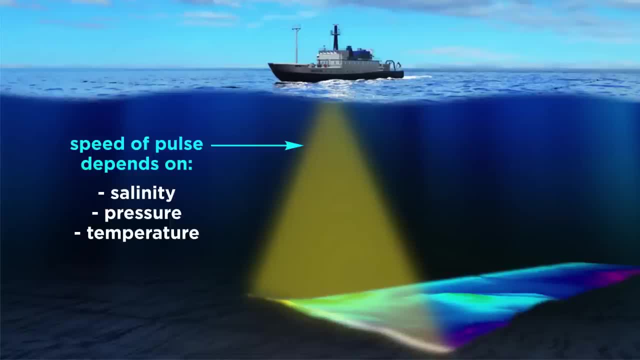 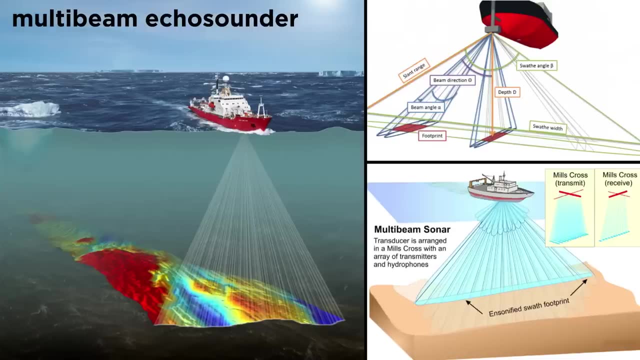 Since the speed of the pulse can vary with ocean water's salinity, pressure and temperature, engineers developed multi-beam echo sounders that send out hundreds of sound pulses and can measure the angle of return from each pulse. With the high angular resolution of the multi-beam echo sounder, scientists can measure ocean. 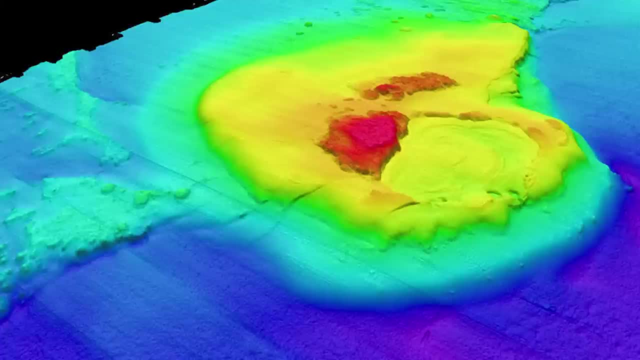 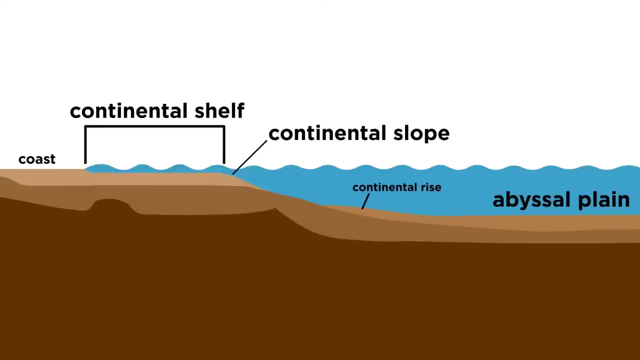 floor features from multiple sides and create a more realistic picture of what these features look like. So what type of landforms are on the ocean floor? For the most part, the very bottom of the ocean floor, called the abyssal plane, is flat and featureless. 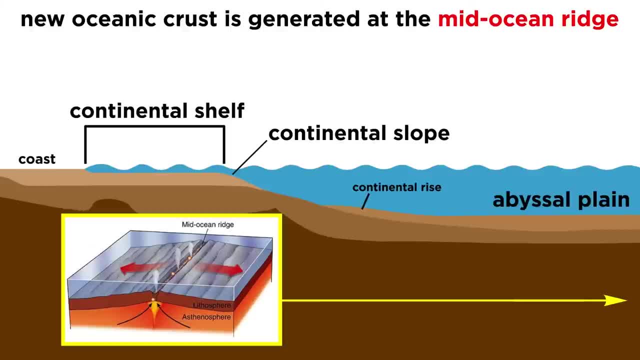 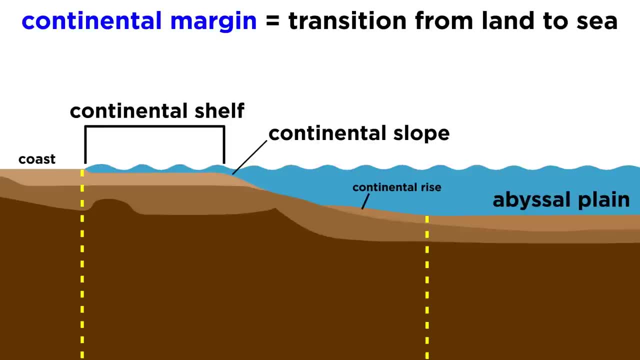 At the center of an ocean basin lies a mid-ocean ridge, where new oceanic crust is being created. On either side of an ocean lies a continental margin, which is simply the transition zone from land to sea. The continental margin is composed of three areas. 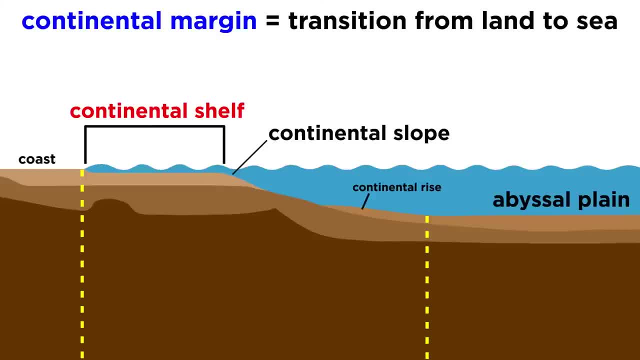 The continental shelf, Which is a gently sloping surface that makes up all shorelines, The continental slope, a steep drop-off that marks the edge of the continental crust, And the continental rise, which is an area where sediment from the continental slope piles up during underwater avalanches called turbidity currents. 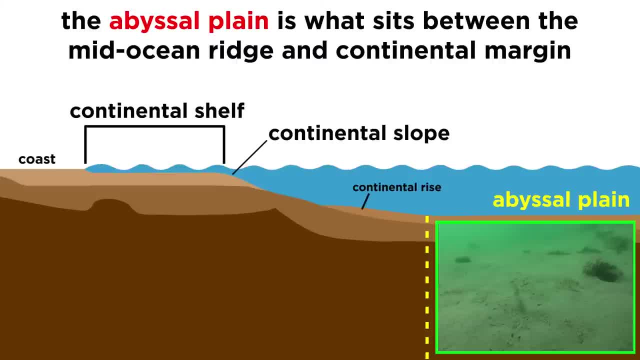 The abyssal plane, which is probably what you imagine when you think of the ocean floor, is located between the mid-ocean ridge and continental margin. The abyssal plane ranges in depth from three to six kilometers and covers 70% of the ocean. 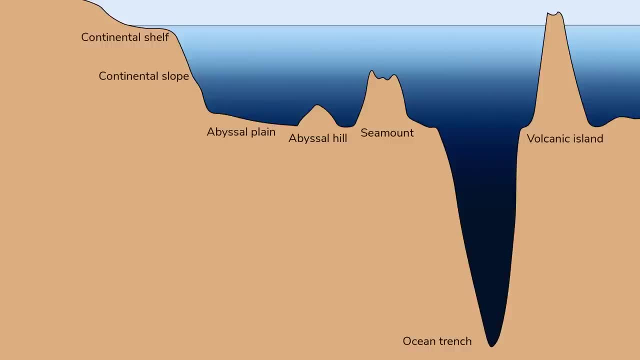 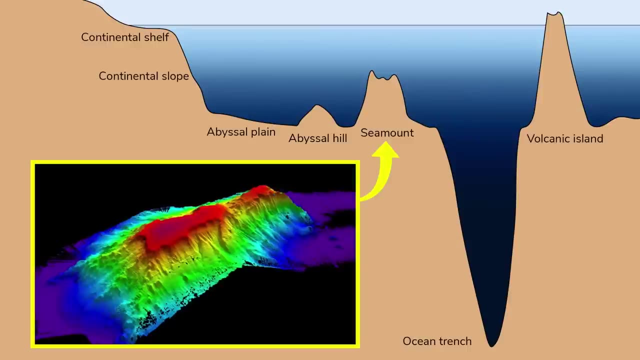 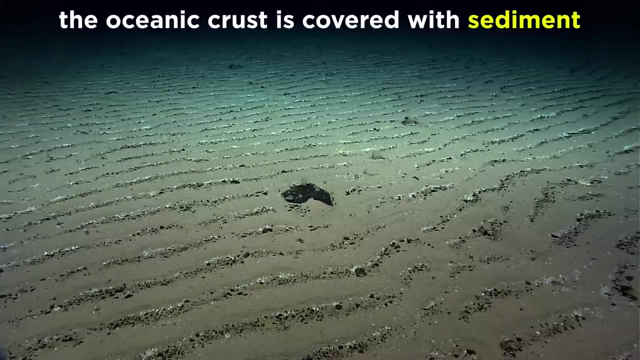 floor. As we mentioned, it is predominantly flat and featureless, with the occasional trench near areas experiencing subduction or volcanic seamount above hot spots, breaking up the monotony. Lying atop the oceanic crust is a thick layer of sediment blanketing the ocean floor, and 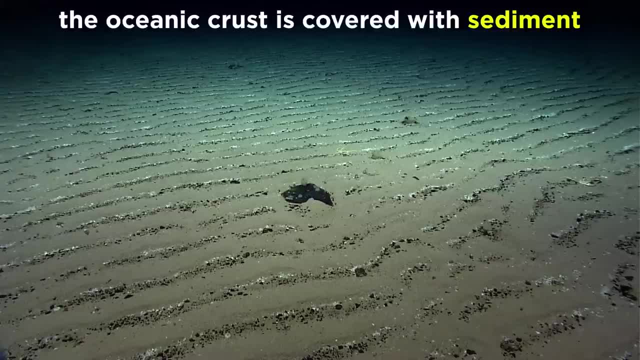 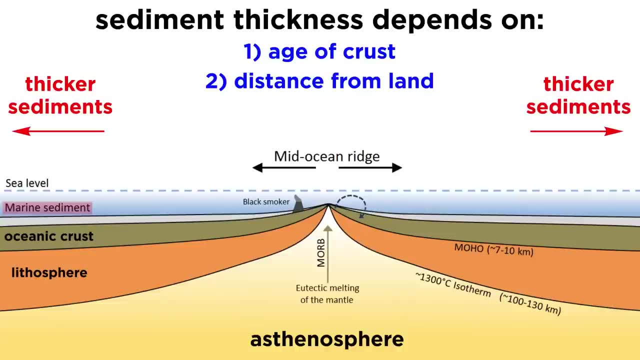 providing a habitat for many types of burrowing organisms. So what's the plan? The sediment thickness varies based mainly on the age of the crust and the distance from land, with the thickest sediments occurring closest to land, where both the sediment supply. 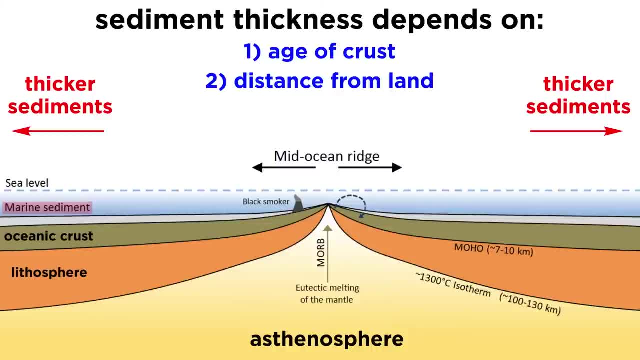 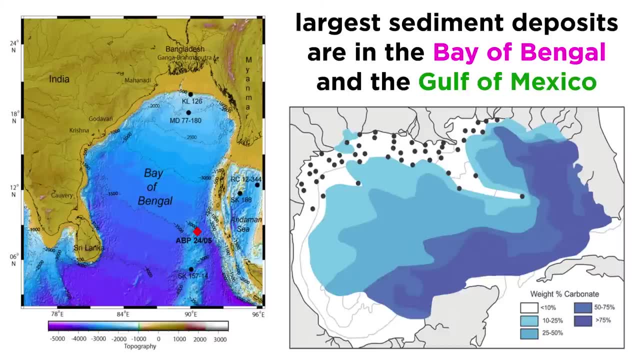 is greatest and oceanic crust is oldest. The largest sediment deposits in today's oceans are in the Bay of Bengal and Gulf of Mexico, where they approach 20 kilometers thick in some spots. For comparison, atop the youngest crust near mid-ocean ridges, sediment is mainly in the 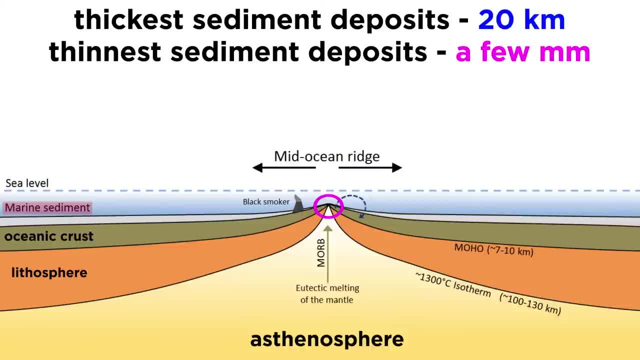 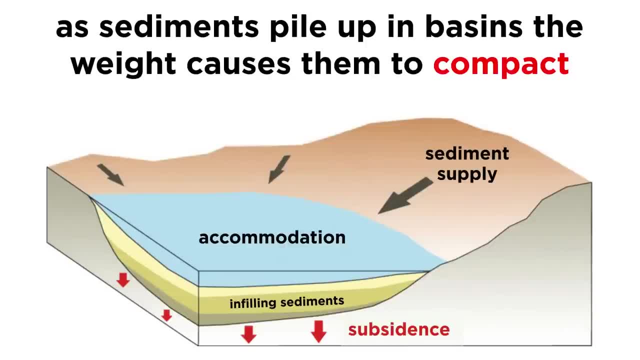 middle of the ocean. This means that sediment is mainly in the middle of the ocean and sediment is mainly in the middle of the ocean. Sediment may only be millimeters thick. As sediment is progressively buried in basins, the weight of the overburden causes the sediment. 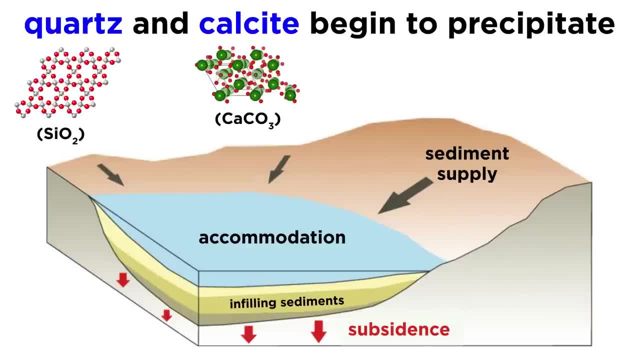 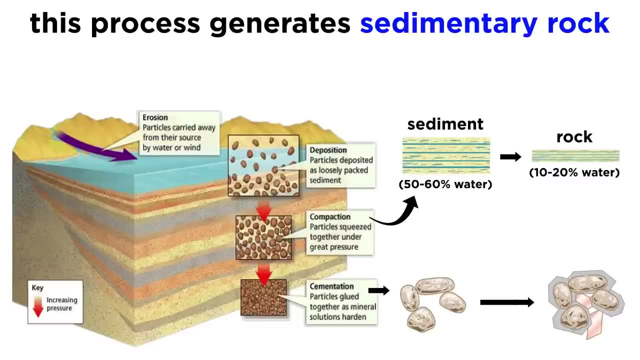 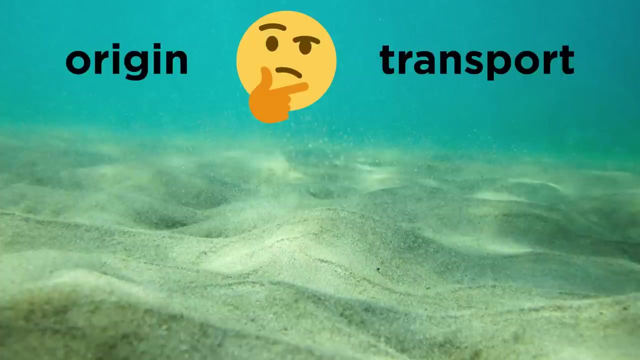 to compact and minerals such as quartz and calcite begin to precipitate from the mineral-laden pore waters, cementing sediment grains together to form a sedimentary rock. This combined process of compaction and cementation is called lithification. To fully understand sedimentary rocks, we need to understand sediments where they 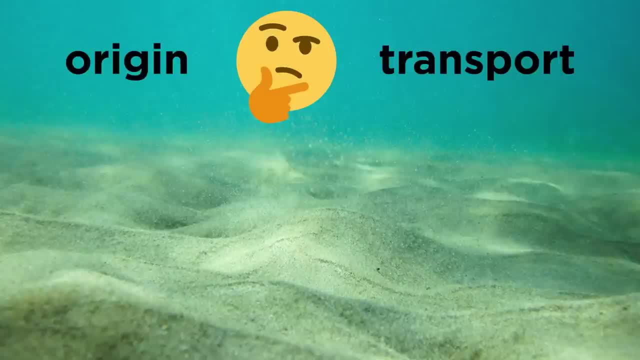 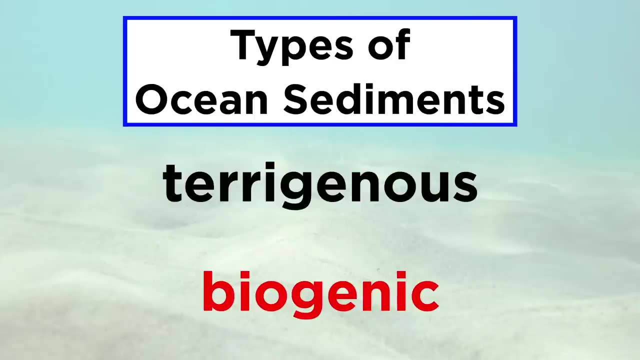 come from, how they are transported and what happens to them during transport. There are two types of sediment found in the ocean: pterygianous and biogenic. Pterygianous sediment is made up of minerals and small rocks that eroded from continental 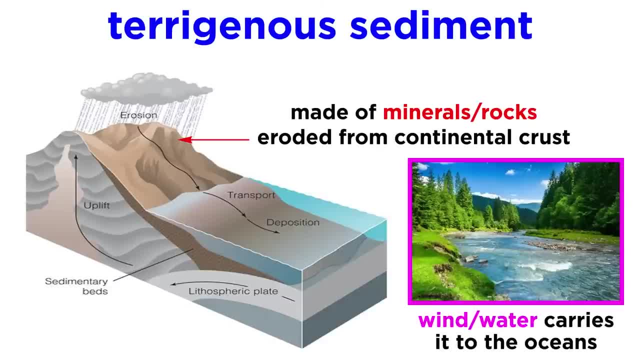 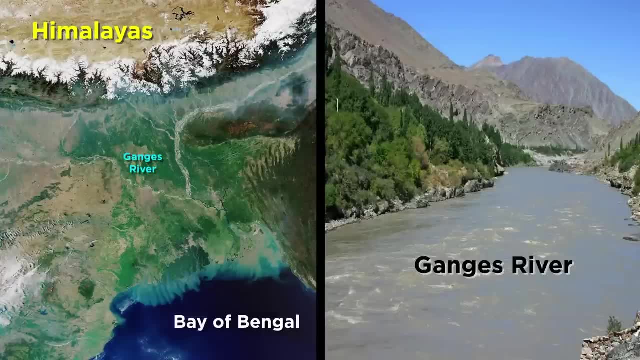 crust, or, more simply, the land, Wind and water- though mainly water- carry sediment from the mountains to the oceans and the mountains to the oceans. The reason that the Bay of Bengal has such a thick sediment layer is that several large river systems are dumping millions of tons of eroded sediment from the rising Himalayas. 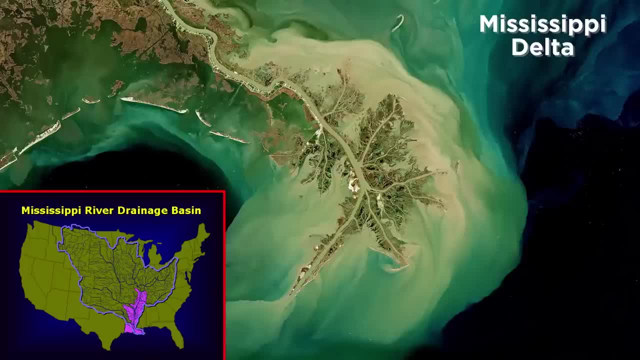 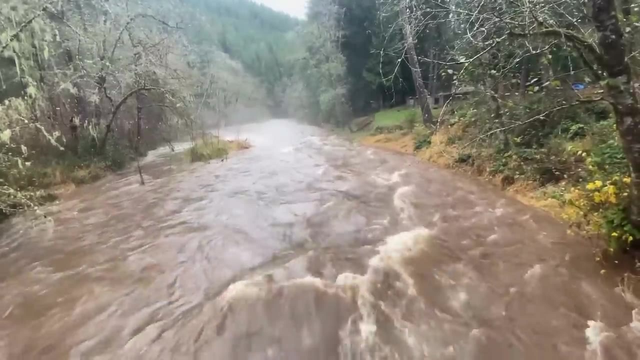 In a similar manner, the Mississippi River carries loads of sediment from the eroding Rockies and Appalachians into the Gulf of Mexico. This is pterygianous sediment. Most pterygianous sediment is transported to the oceans during large storms and floods, when river flow is fastest. 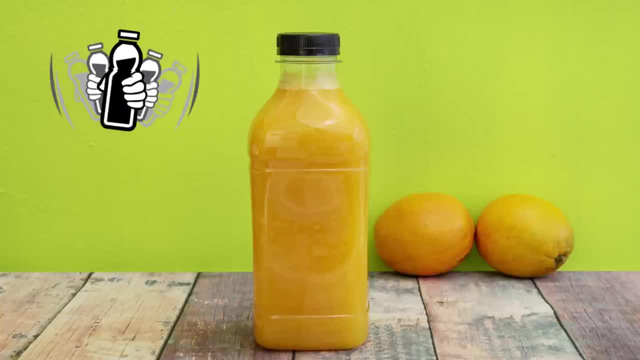 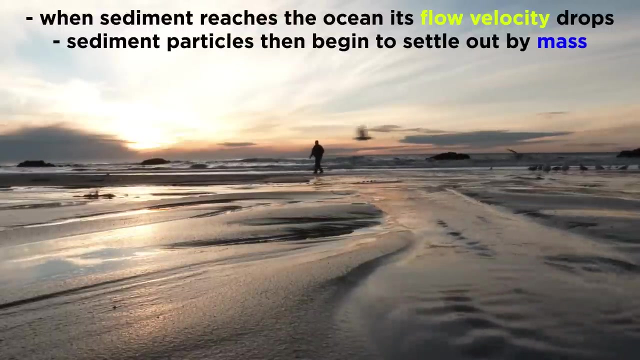 This is the same reason why you probably shake your orange juice before pouring a glass. Shaking it increases its velocity, allowing the juice to lift the pulp into suspension. Once the sediment reaches the open ocean, flow, velocity drops and it begins to settle out by mass. 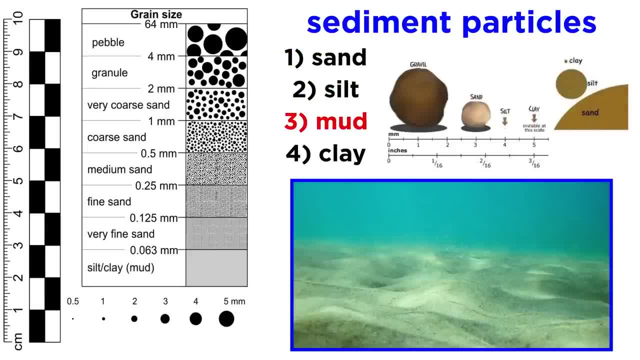 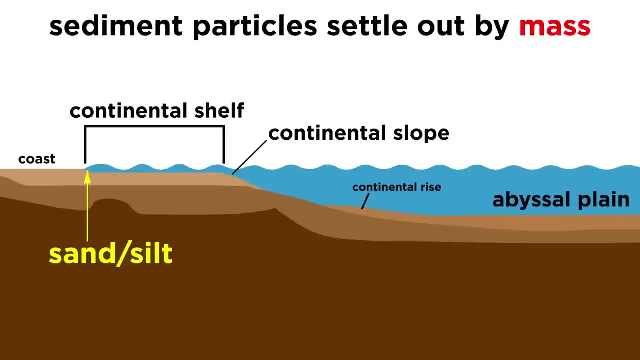 Sand settles out first, followed by silt, then mud, with clay being the last to settle out. Sand is sometimes remaining suspended in the ocean for hundreds to thousands of years. Since the largest grains settle out first, sand and silt are only found near the shoreline. 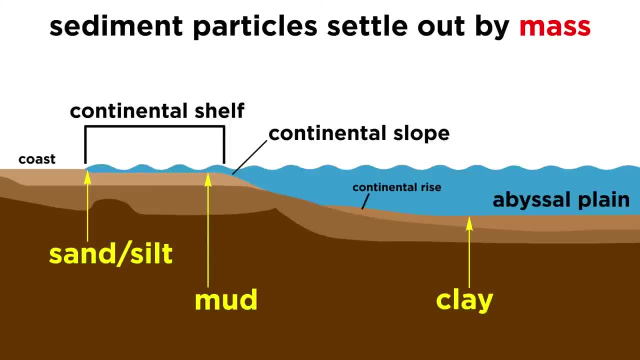 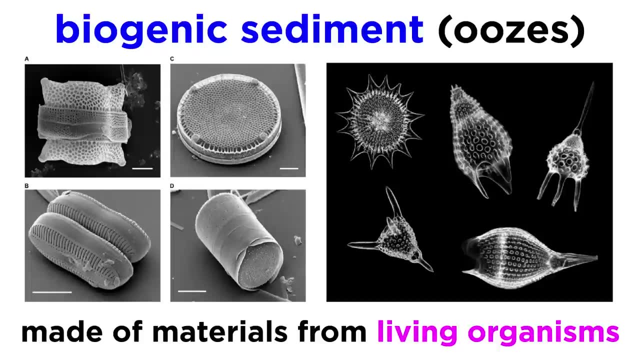 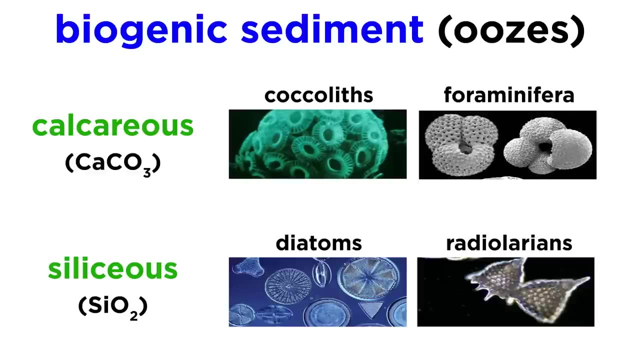 with mud accumulating further offshore and only the smallest clay particles reaching the open ocean, slowly accumulating on the abyssal. plain Biogenic sediments, or oozes, are made of materials created by living organisms. There are two categories of sediment. 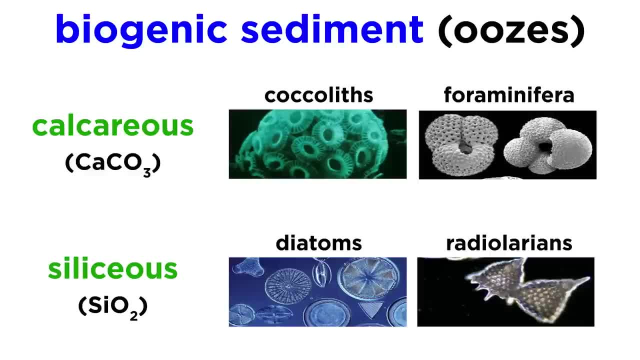 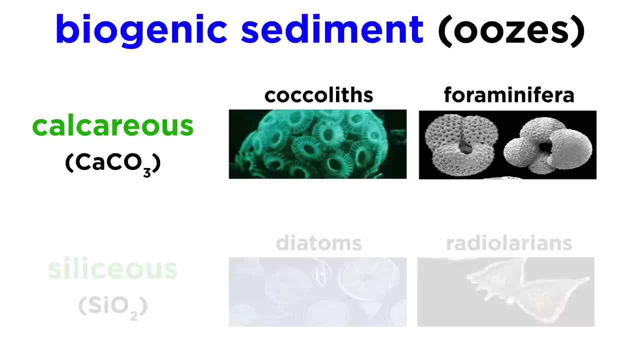 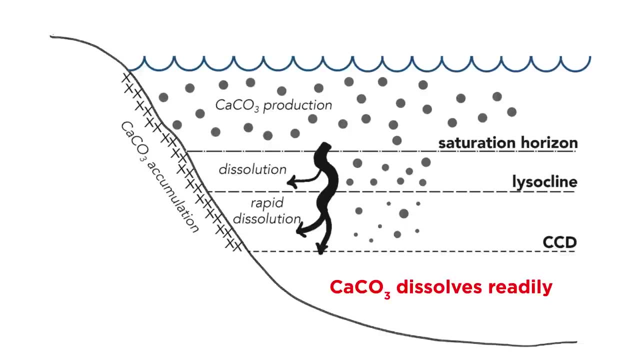 There are two categories of biogenic sediment that accumulate on the ocean floor: Calcareous and siliceous. Calcareous biogenic sediments are comprised of the calcium carbonate skeletons from single-celled marine organisms like foraminifera. However, since calcium carbonate dissolves readily in colder, deeper water, calcareous 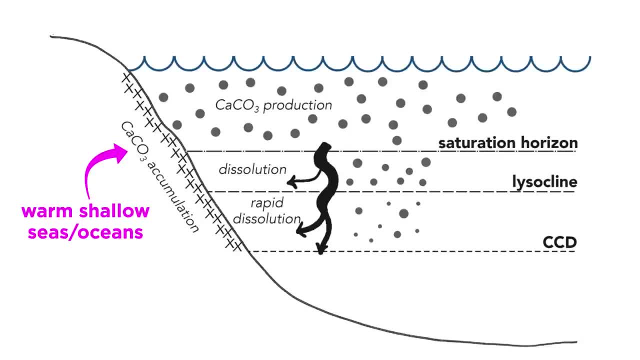 oozes are primarily found in warm shallow seas. The depth at which calcium carbonate starts to dissolve is the depth at which the ocean starts to sink in. Calcareous oozes are primarily found in warm shallow seas. The depth at which calcium carbonate starts to sink in is the depth at which the ocean. 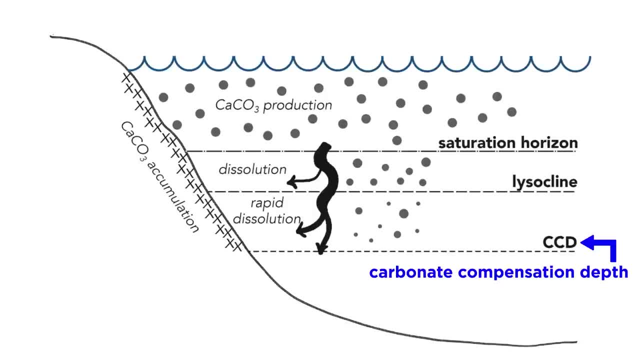 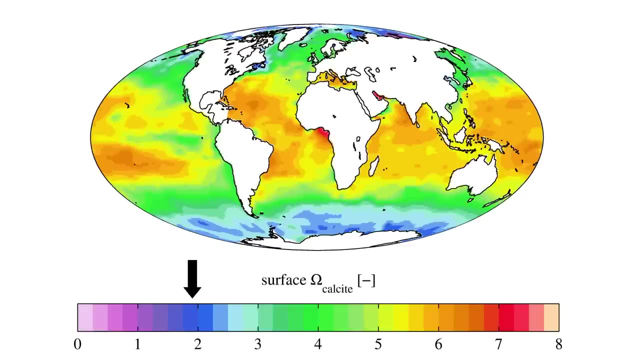 starts to dissolve in ocean water is called the carbonate compensation depth, abbreviated as CCD. Since the CCD is a function of temperature and seawater chemistry, its exact depth varies, being deeper in equatorial regions and shallower near the poles. By mapping this depth across the ocean, scientists created the lysocline, which shows how the 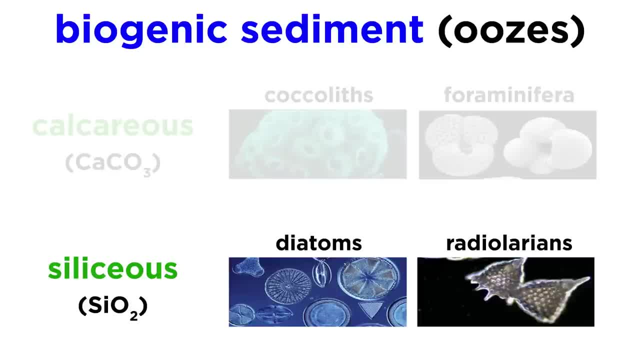 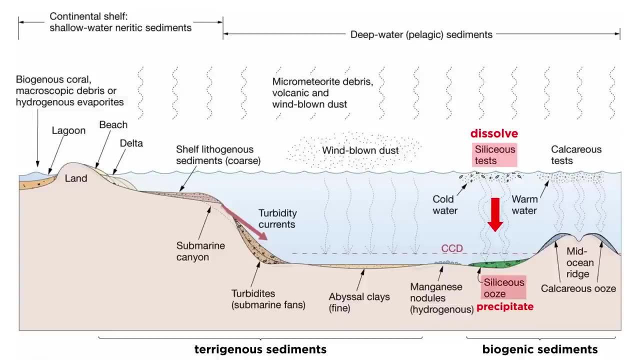 CCD changes with location. Calcareous biogenic sediments are made of the silica skeletons from single-celled marine organisms like diatoms and radiolarians. Siliceous oozes are essentially the opposite of calcareous oozes, in that the silica tends. 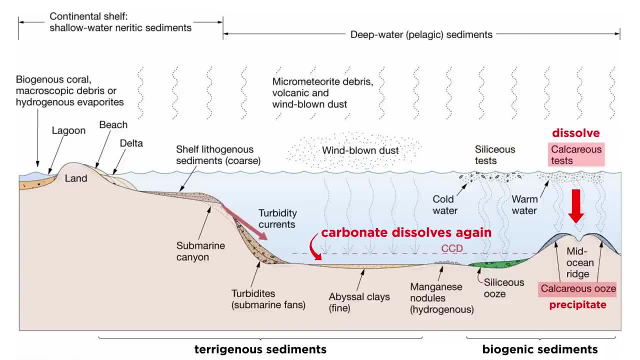 to dissolve rapidly in the shallow ocean, whereas carbonate rapidly dissolves in deep water, as we mentioned. Given the high solubility in seawater, siliceous oozes only form in areas where diatom and radiolarians are thriving and sedimentation can exceed dissolution. 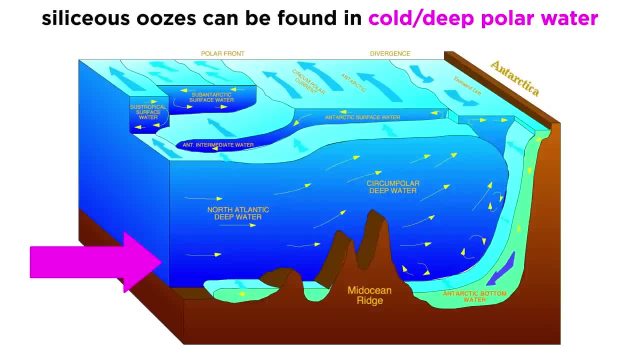 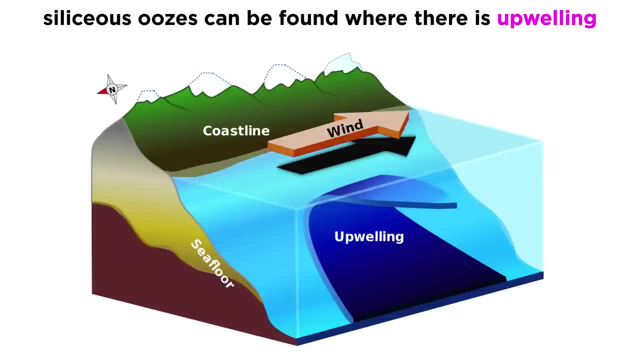 Unlike the calcareous, siliceous oozes are likely to be found in the cold deep water, at the poles or in areas where upwelling occurs. Upwelling is a process where strong winds and the Earth's rotation cause shallow waters. 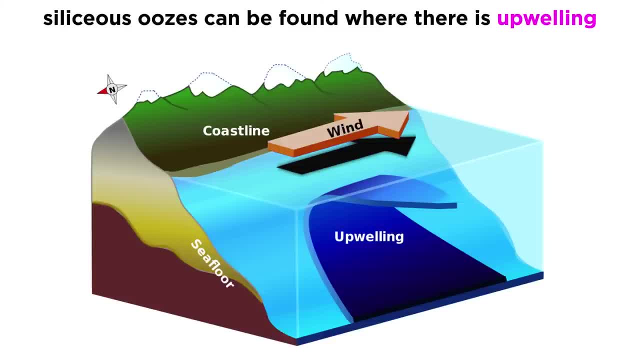 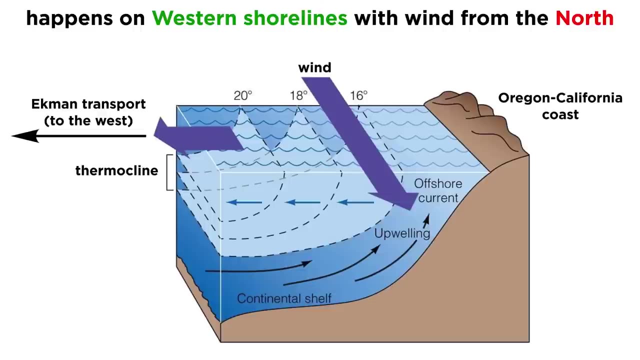 to diverge, allowing deep cold water to rise to the surface, filling the space created by the diverging surface waters. Upwelling tends to occur along western shorelines, where winds blow from the north which, when modified by the Coriolis force, cause an ocean current that moves away from land or 90 degrees.